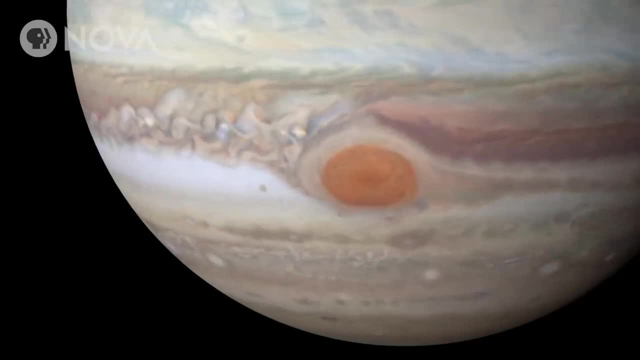 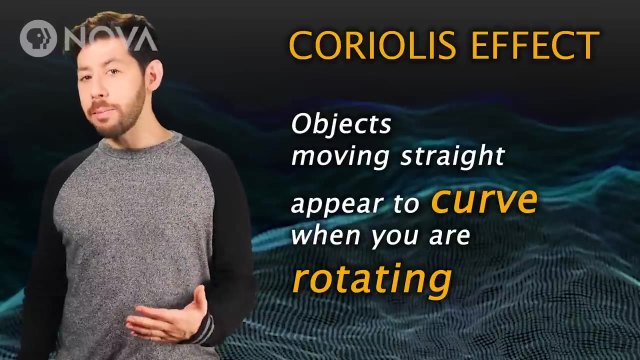 effect is what makes hurricanes spin, and it's the reason why Jupiter's great red spot is spinning the way that it is. So what is the Coriolis effect? Well, it's what makes a hurricane spin. What happens when objects moving in a straight line appear to curve? because you are rotating? 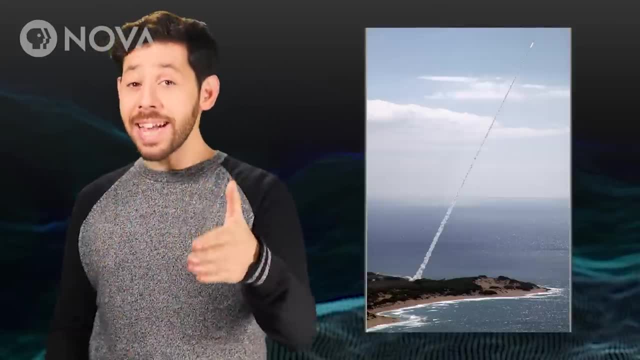 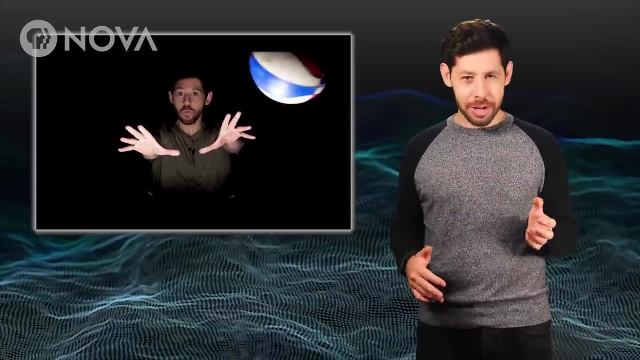 And it affects all kinds of things. It bends the paths of missiles and sniper shots, But how does it work and how does it create hurricanes? Right now it seems like the ball's curving, But let's take a look at what's really happening. My friends and I put together this little experiment using a 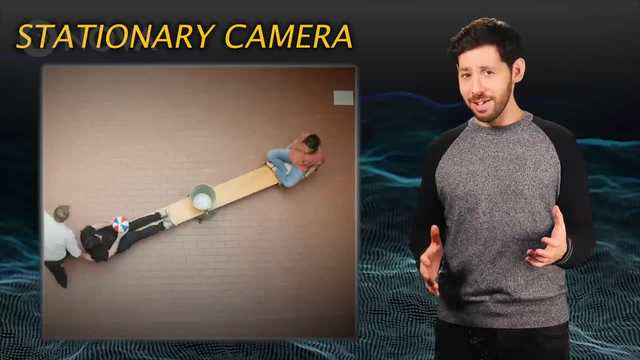 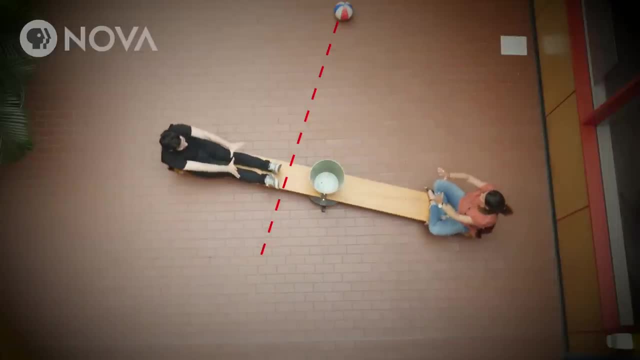 sort of spinning seesaw Here. the camera's standing still, It's just hanging from the ceiling And watch what happens From the moment the ball is moving, it turns into a curve and it turns into a rotation. Once the ball leaves my hand, it's just going straight. Let's watch that again, frame by frame. 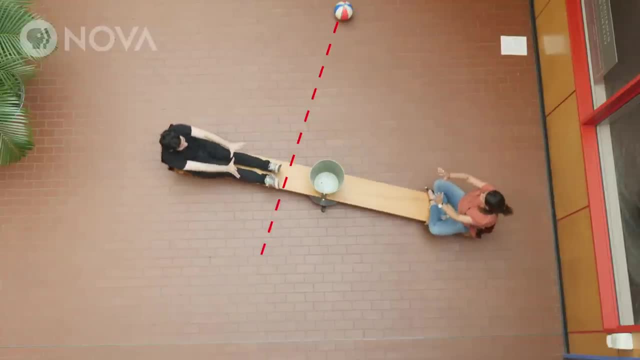 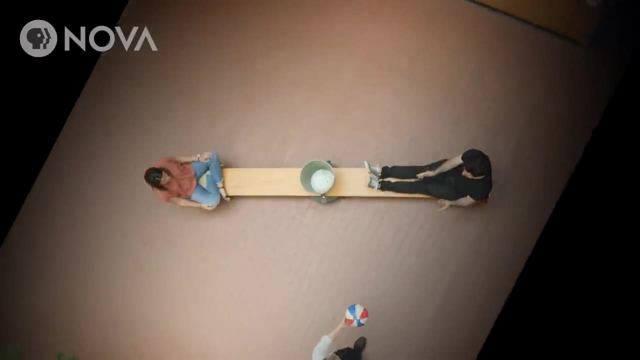 Keep your eye on the ball, You can see it travels in a perfectly straight line. But what if you're spinning with the seesaw? Look at what happens when you rotate the footage. so the seesaw stays sideways and everything moves around it. Now let's follow the path of the ball again, but 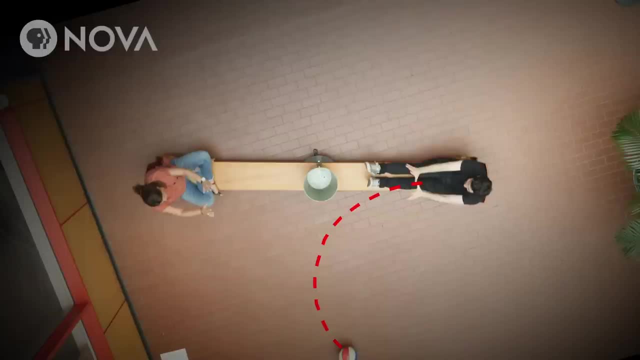 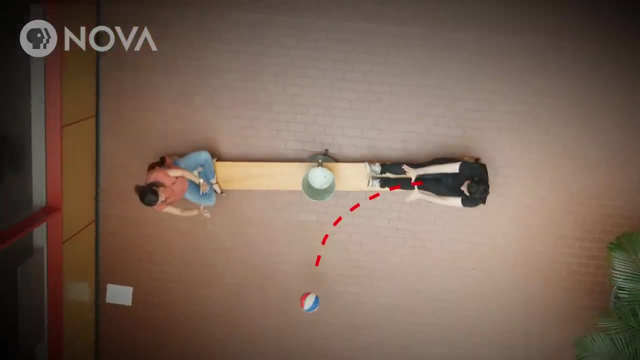 from this new perspective, The trajectory looks completely different. Now let's watch this one frame by frame. From this rotating perspective, it totally looks like the ball is curving. That's crazy, because you already saw that exact same throw. Watch it again on the left. 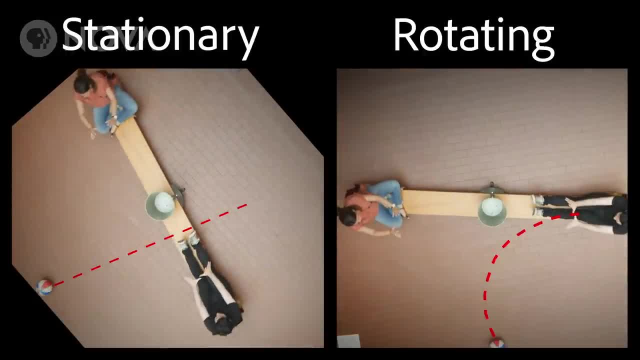 The ball is going straight, but on the right, when you're rotating with a see saw, the ball really looks like it's curving. You might be thinking: why should I care? I don't spend a lot of time on a spinning see saw or on a. 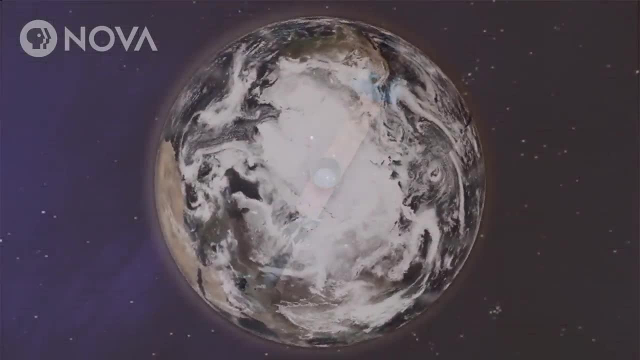 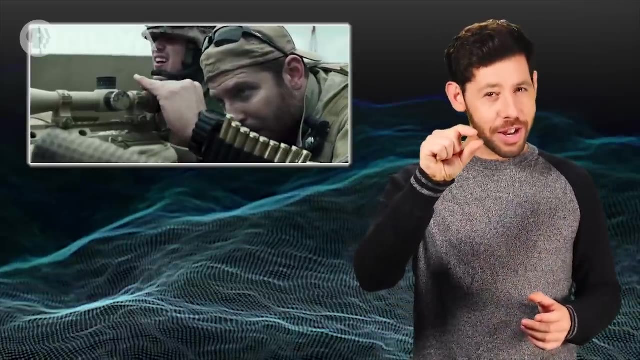 Merry-go-round. But let's try something else. Maybe a maze, Or you can see a ball flying around the board now, But you kind of are on a merry-go-round. The Earth is constantly spinning. Have you ever seen someone in a movie making fine adjustments on their gun? 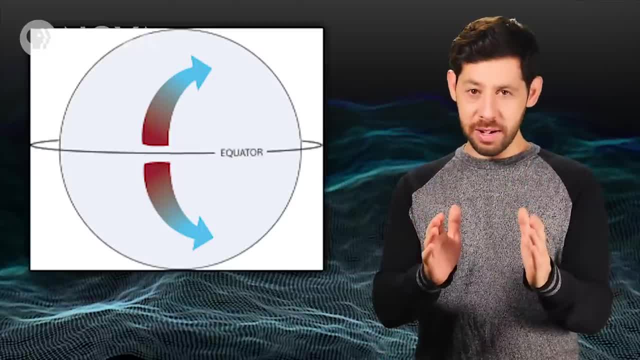 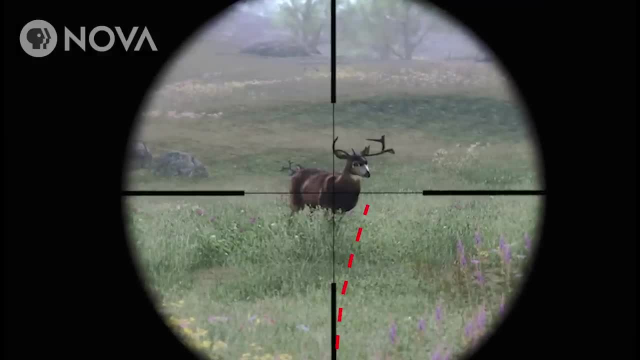 Well, one effect they're correcting for is the Coriolis effect. The longest sniper shot, which was over 3,000 yards, would have had to correct for a one-foot deviation due to the Coriolis effect. So how does the Coriolis effect create hurricanes?